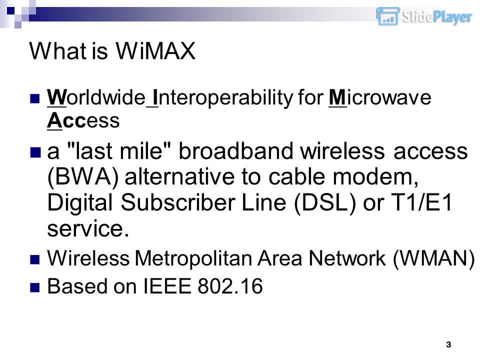 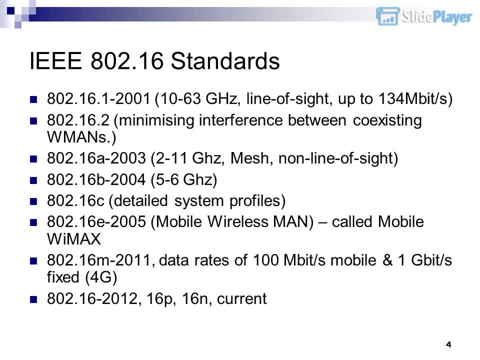 Wireless Metropolitan Area Network, WMAN, Based on IEEE 802.16. IEEE 802.16 Standards. 802.16.1-2001, 10-63 GHz Line of Sight up to 134 Mbps. 802.16.2- Minimizing interference between coexisting WANs. 802.16a 2003,. 2-11 GHz Mesh- non-line-of-sight. 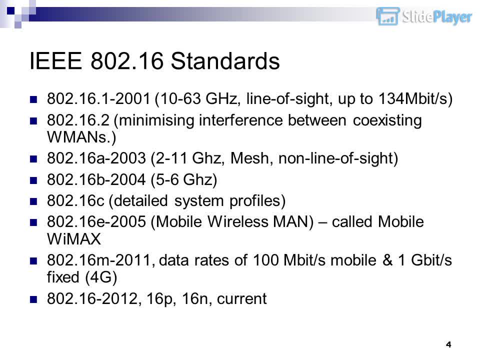 802.16b 2004,. 5-6 GHz. 802.16c- Detailed System Profiles. 802.16e-2005, Mobile Wireless Man called Mobile WiMAX. 802.16m-2011, Data Rates: of 100Mbps Mobile and 1Gbps Fixed 4G. 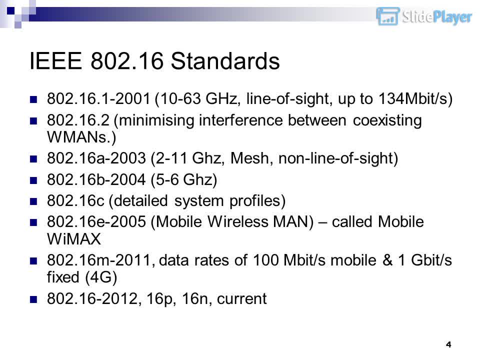 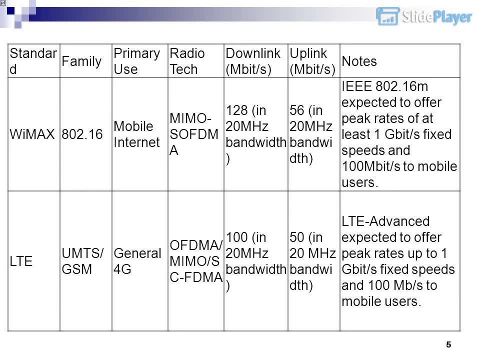 802.16-2012, 16p, 16n. Current Standard Family Primary Use. Radiotech Downlink- mbit-slash-s Uplingle, mbit-slash-s Notes. WiMAX 802.16- Mobile Internet MIMO, SOFMA. 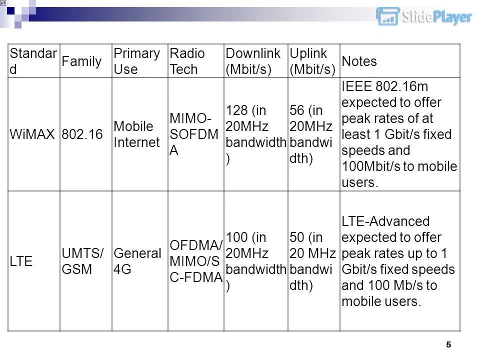 128, in 20MHz Bandwidth, 56, in 20MHz Bandwidth. IEEE 802.16m expected to offer peak rates of at least 1Gbps, fixed speeds and 100Mbps to mobile users: LTE, UMTS-GSM. 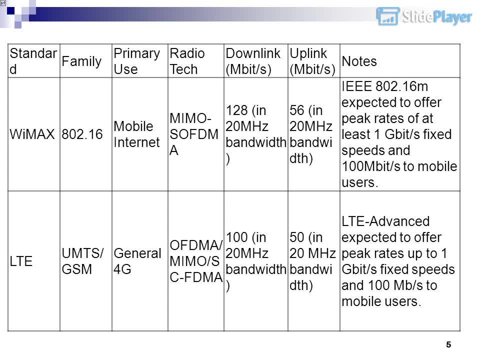 General 4G OFMA-slash-MIMO-slash-S-A-F-DMA- 100, in 20MHz Bandwidth. 50, in 20MHz Bandwidth. LTE Advanced, Expected to offer Peak Rates up to 1Gbps, fixed speeds and 100Mbps to mobile users. 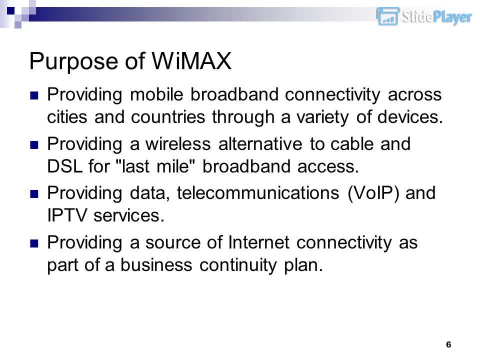 Purpose of WiMAX. Providing Mobile Broadband Connectivity across cities and countries through a variety of devices. Providing a wireless alternative to cable and DSL for last-mile broadband access. Providing data telecommunications, VoIP and IPT-ion IPTV services. Providing a source of internet connectivity. 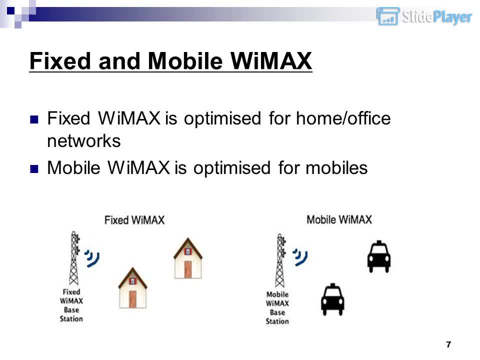 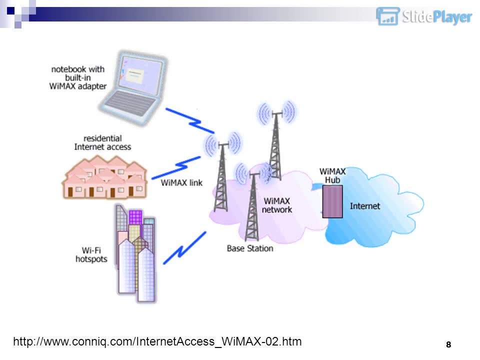 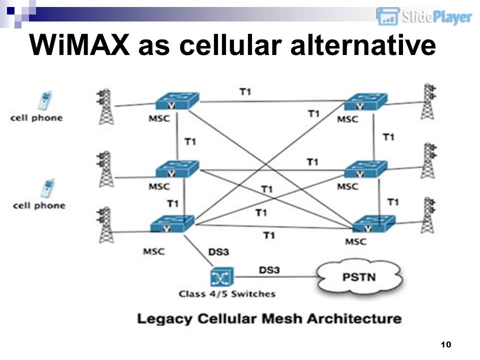 as part of a business continuity plan. Fixed and mobile WiMAX. Fixed WiMAX is optimized for home-slash-office networks. Mobile WiMAX is optimized for mobiles: http//wwwconiccom/internet-access-underscore-wimax02.htm. Fixed WiMAX Architecture. WiMAX as Cellular Alternative. 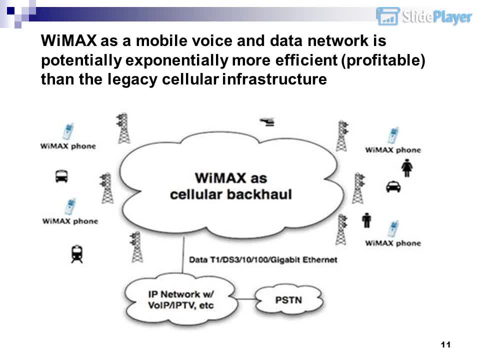 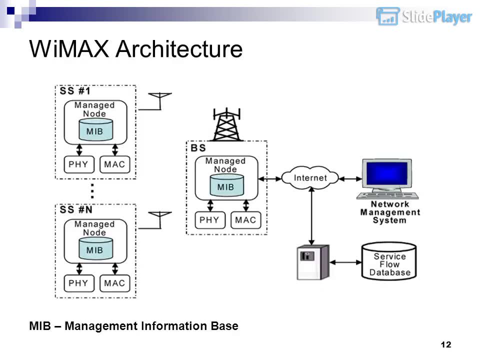 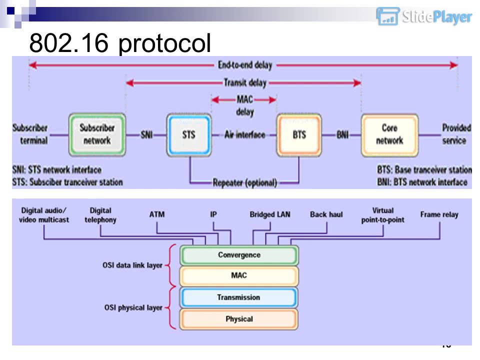 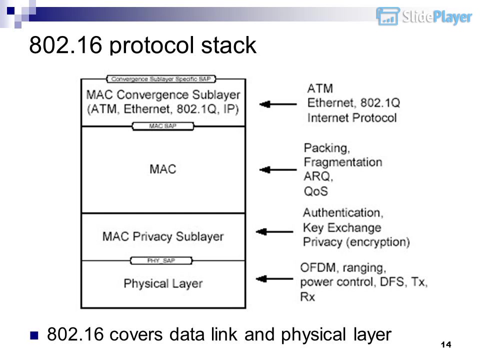 WiMAX as a mobile voice and data network is potentially exponentially more efficient, profitable than the legacy cellular infrastructure. WiMAX Architecture, MIB Management Information Base- 802.16 Protocol- 802.16 Protocol- Stack 802.16 Covers Data Link and Physical Layer. 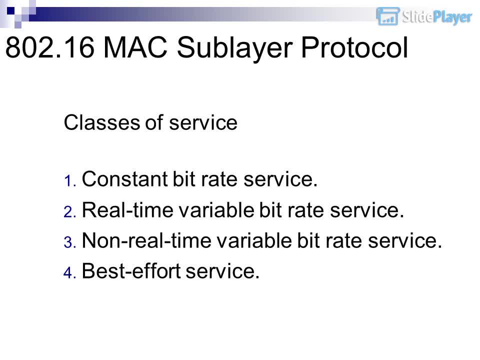 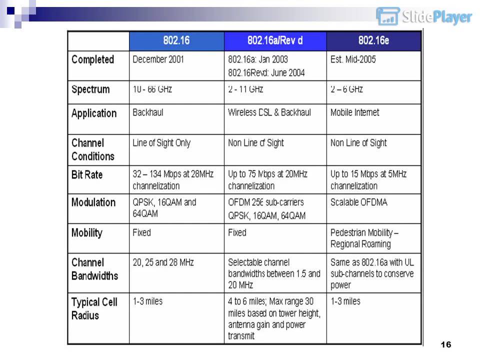 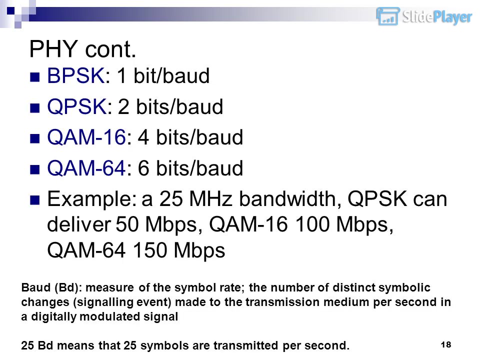 802.16 MAC Sublayer Protocol. Classes of Service. Constant Bitrate Service. Real-Time Variable Bitrate Service. Non-Real-Time Variable Bitrate Service. Best Effort Service. Best Effort Service. Physical Layer PHY Cont BPSK 2 bits slash board CAM16. 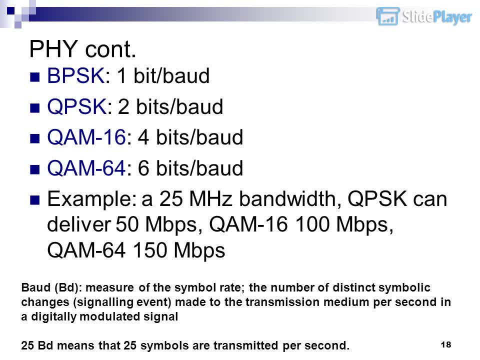 4 bits slash board. Example A: 25 MHz bandwidth: QPSK can deliver 50 Mbps. QPSK can deliver 50 Mbps. QPSK can deliver 50 Mbps per second. QPSK can deliver 20 Mbps per second. QPSK can deliver 55 Mbps per second. 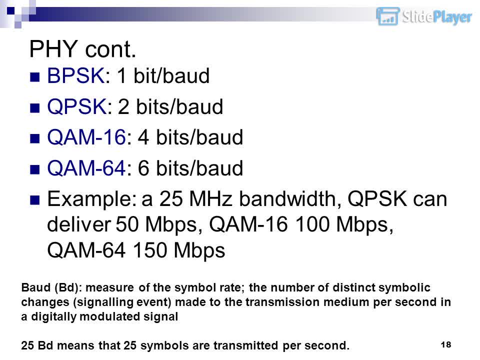 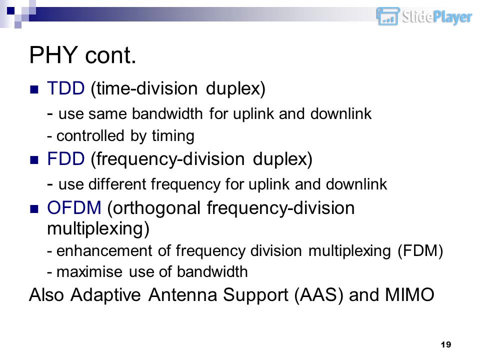 QPSK can deliver 50 Mbps per second. Bissano duplex: Use same bandwidth for uplink and downlink Controlled by timing. FDD frequency division duplex: Use different frequency for uplink and downlink. OFDM orthogonal frequency. 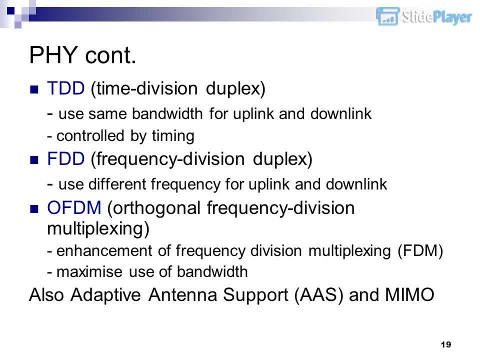 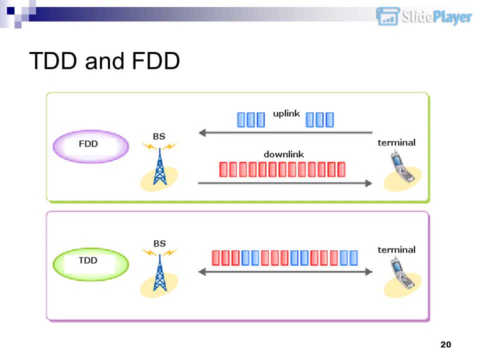 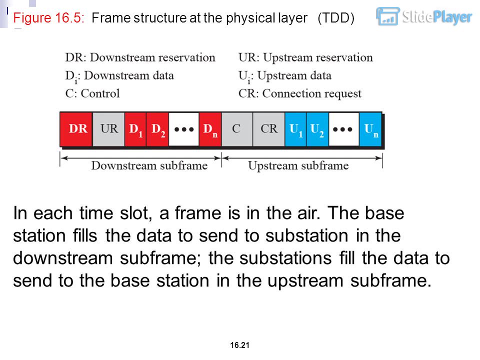 division, multiplexing, Enhancement of frequency division multiplexing, FDM- Maximize use of bandwidth. Also, adaptive antenna support, AS and MIMO, TDD and FDD. Figure 16.5, frame structure at the physical layer. TDD: In each time slot a frame is in the air. The base. 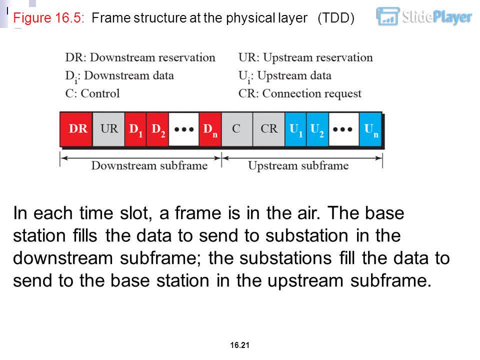 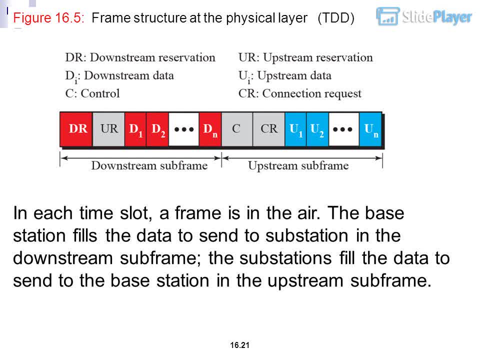 send to substation in the downstream subframe. The substations fill the data to send to substation in the downstream subframe. How bidirectional communication can be achieved in WiMAX using a frame in following figure 1.. Let us assume that WiMAX uses only TDM. Let us assume that 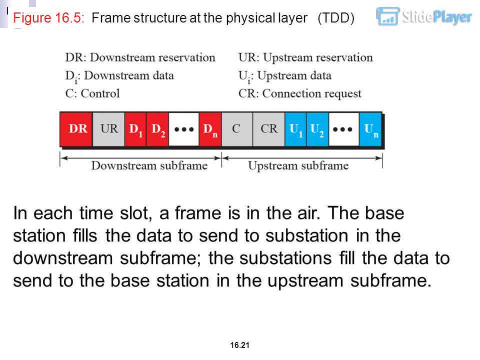 WiMAX uses only TDM. In each time slot a frame is in the air. The base station fills the data to send to substation in the downstream subframe. The substation fills the data to substations. fill the data to send to the base station in the upstream subframe. 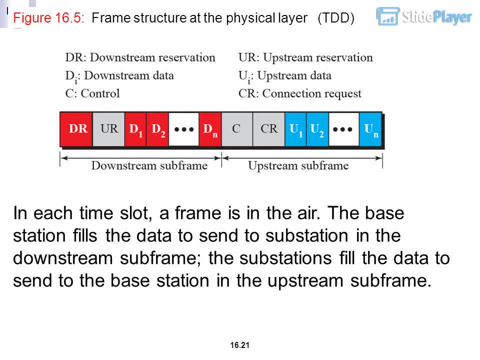 Let us give a very simplified example to make the point clear. Assume that the time slot is 1 minute and the communication is instantaneous. This means in each minute there is a frame in the air. 1. During the first half of each minute, the base station is sending data to the substations and the substations 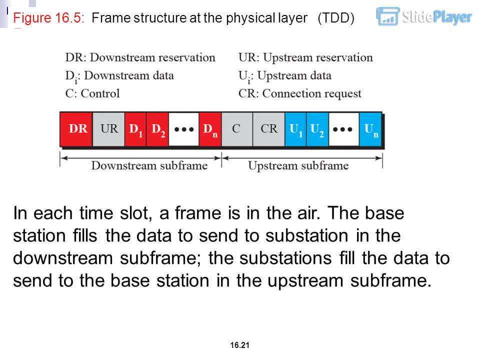 are receiving data from the base station. 2. During the second half of each minute, the substations are sending data to the base station and the base station is receiving data from the substations. 16. OFDM uses bandwidth which is not. 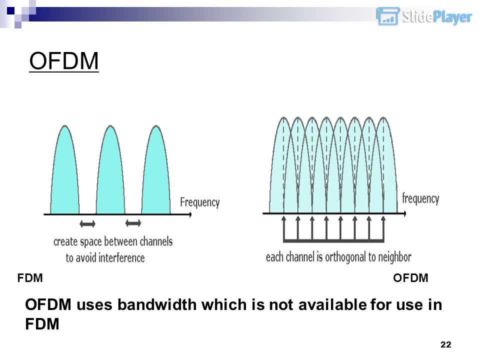 available for use in FDM-FDM. WIMAX FDM-FDM uses bandwidth which is not available for use in FDM-FDM. WIMAX FDM uses bandwidth which is not available for use in FDM-FDM. WIMAX FDM uses bandwidth which is not available to use in FDM-FDM. 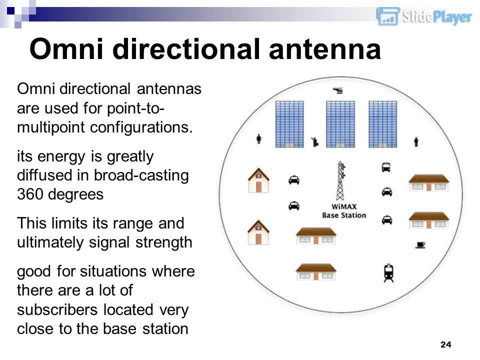 WIMAX FDM uses bandwidth which is not available to use in FDM-FDM 16. Omni-directional antennae. Omni-directional antennae are used for point-to-multipoint configurations. Its energy is greatly diffused in broadcasting 360-degrees. This limits its range and ultimately signals. 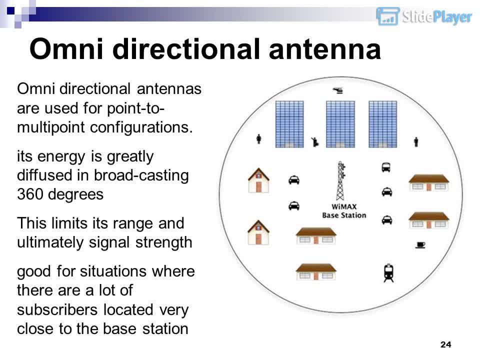 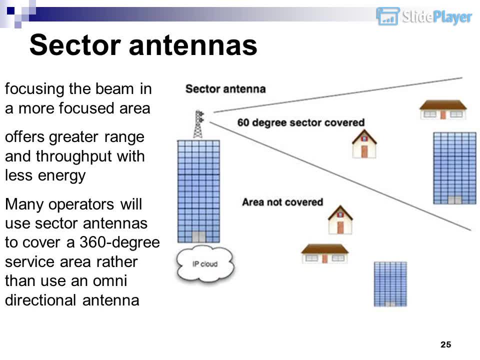 strength Good for situations where there are a lot of subscribers located very close to the base station Sector antennas. focusing the beam in a more focused area offers greater range and throughput with less energy. Many operators will use sector antennas to cover a 360-degree service area rather than use an omnidirectional antenna. 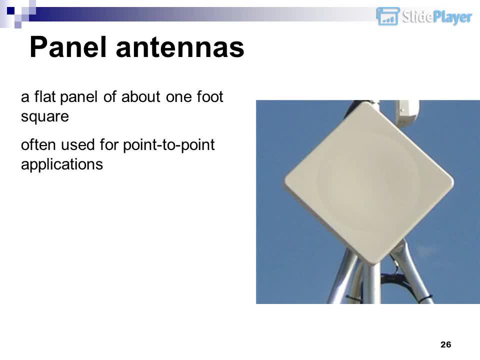 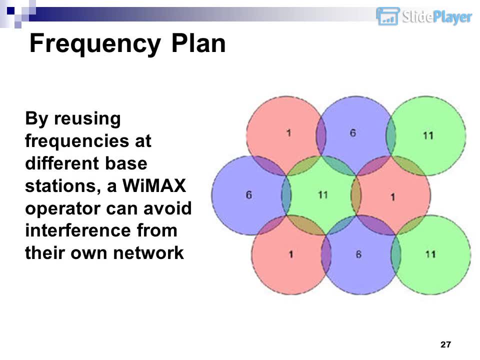 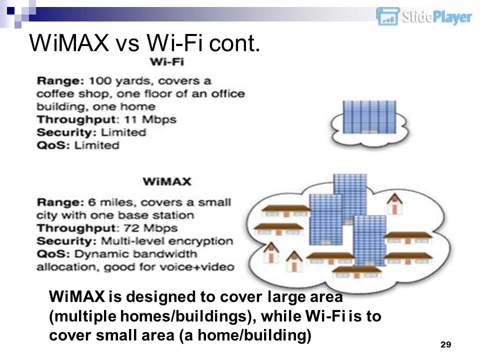 Panel. antennas are flat panel of about 1 foot square often used for point-to-point applications. Frequency plan: By reusing frequencies at different base stations, a WiMAX operator can avoid interference from their own network. WiMAX vs Wi-Fi. WiMAX vs Wi-Fi can't. 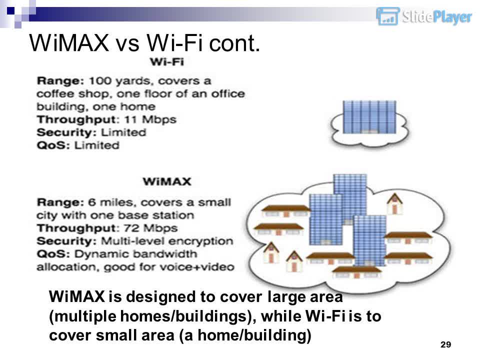 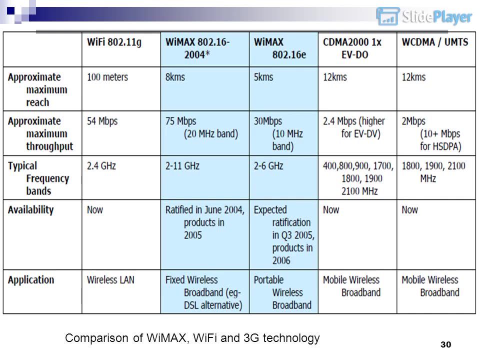 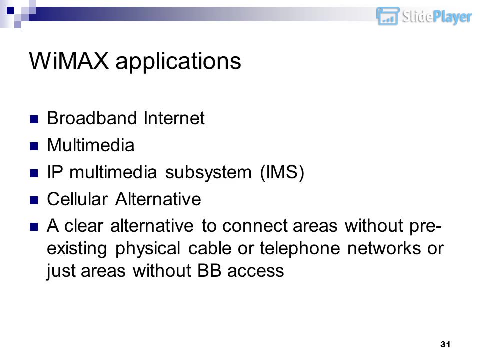 WiMAX is designed to cover large area, while Wi-Fi is to cover small area. Comparison of WiMAX, Wi-Fi and WiMAX. Comparison of WiMAX, Wi-Fi and WiMAX WiMAX applications- broadband internet, multimedia, IP, Multimedia Subsystem, Cellular alternative- A clear alternative to connect areas without pre-existing physical cable or telephone networks, or just areas without BB access. 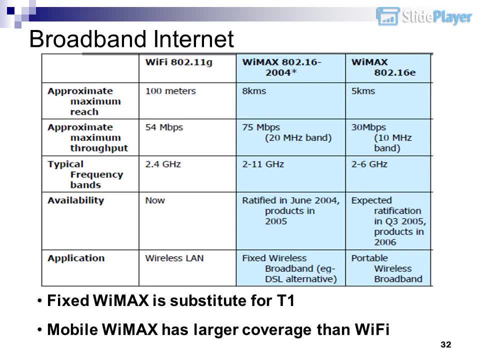 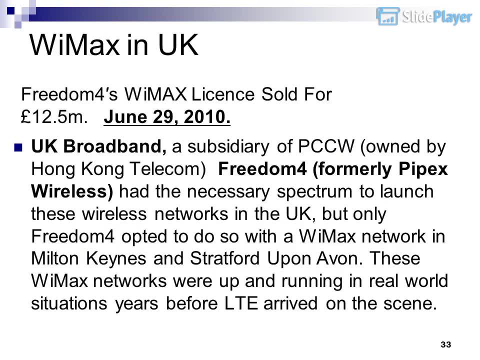 Broadband Internet Fixed WiMAX is substitute for T1 Mobile. WiMAX has larger coverage than Wi-Fi WiMAX. in UK, Freedom 4's WiMAX license sold for £12.5 million. June 29, 2010, UK Broadband, a subsidiary of PCCW owned by Hong Kong Telecom. 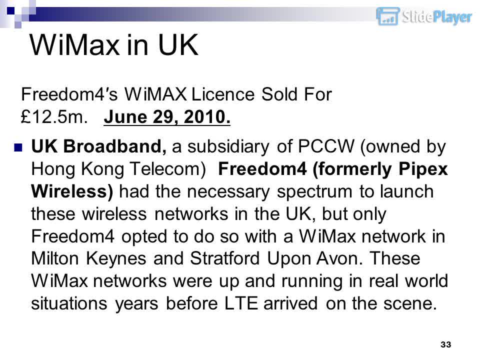 Freedom 4 had the necessary spectrum to launch these wireless networks in the UK, but only Freedom 4 opted to do so with a WiMAX network in Milton Keynes and Stratford-upon-Avon. These WiMAX networks were up and running in real-world situations years before LTE arrived on the scene. 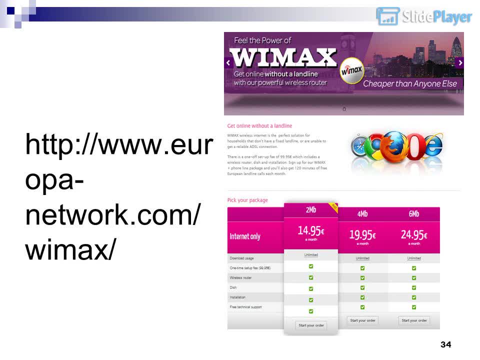 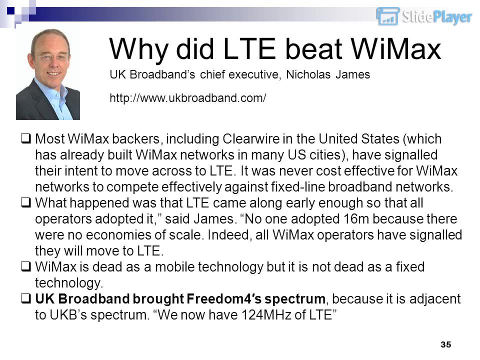 http//wwweuropanetworkcom/wimax/ Why did LTE beat WiMAX? UK Broadband's Chief Executive, Nicholas James, said. Nicholas James, http//wwwukebroadbandcom/ Most WiMAX backers, including Clearwire in the United States. 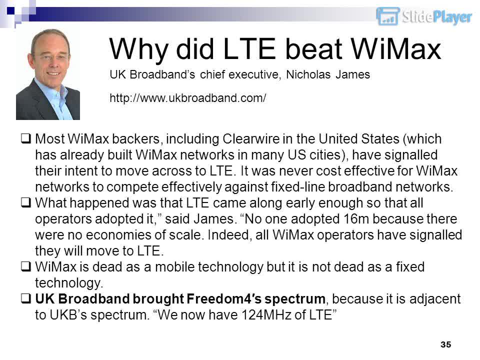 which has already built WiMAX networks in many US cities, have signalled their intent to move across to LTE. It was never cost-effective for WiMAX networks to compete effectively against fixed-line broadband networks. What happened was that LTE came along early enough so that all operators adopted it, said James. 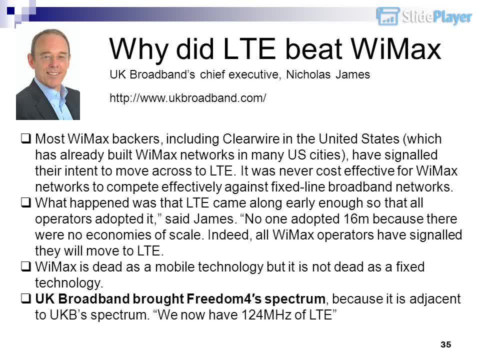 No one adopted 16 meters because there were no economies of scale. Indeed, all WiMAX operators have signalled they will move to LTE. WiMAX is dead as a mobile technology, but it is not dead as a fixed technology. UK Broadband brought Freedom 4's spectrum. 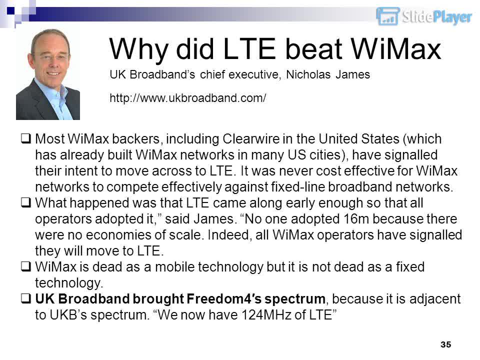 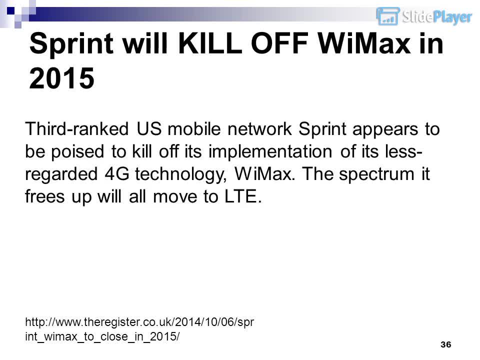 because it is adjacent to UKB's spectrum. We now have 124 MHz of LTE. Sprint will kill off WiMAX in 2015.. Third-ranked US mobile network, Sprint appears to be poised to kill off its implementation of its less-regarded 4G technology, WiMAX.